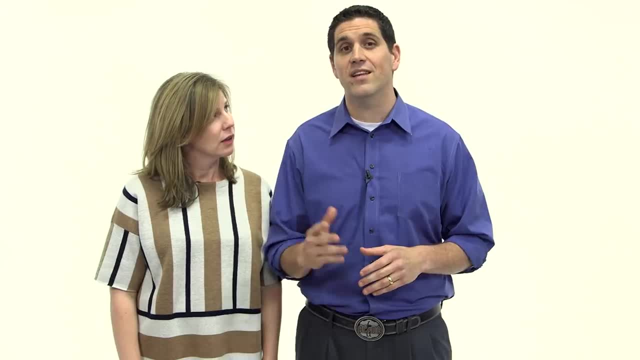 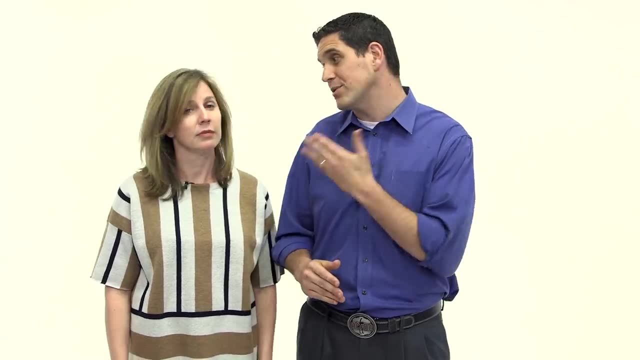 But it doesn't have to be that complicated. Remember, economics is the study of scarcity and choices. We have limited resources, so we need a way to analyze the best way to use them. We need economics to make wise decisions in the future, but it also helps us understand. 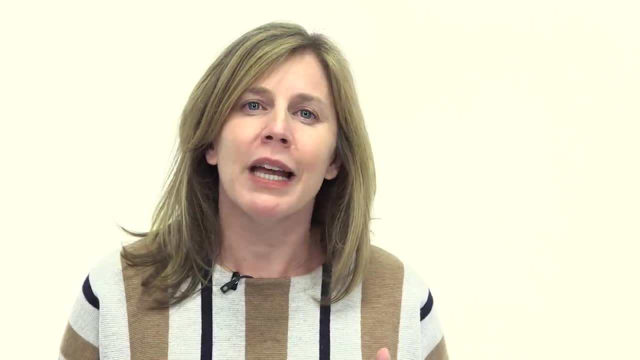 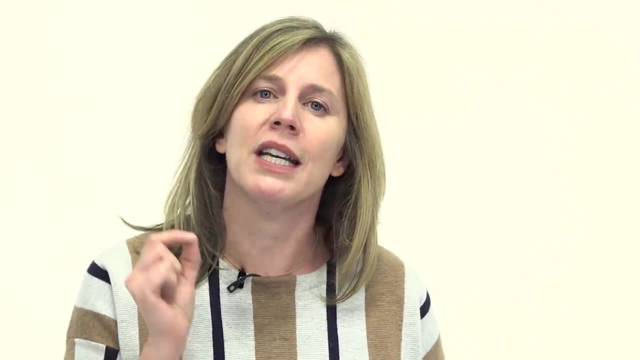 the past. Most empires, wars and human endeavors can be explained using economics. All you have to understand is who wanted what. The American Civil War wasn't just about freedom. It was fought because southern states wanted to keep using cheap slave labor. It was economics. 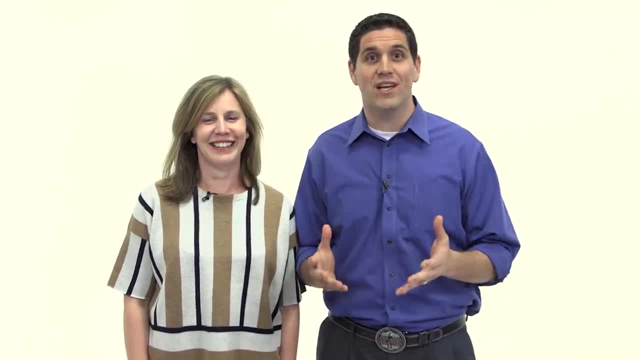 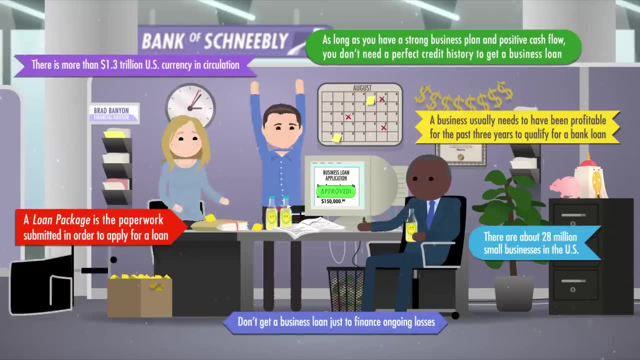 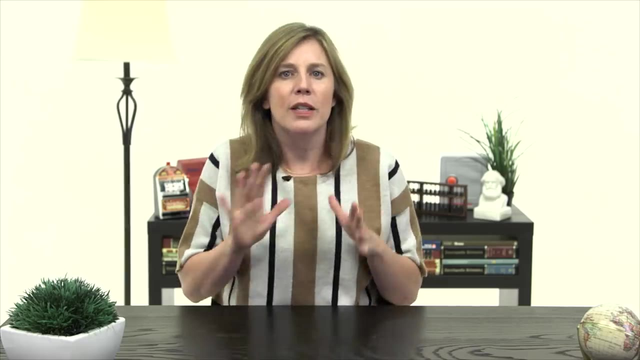 Econ can explain so much about the world and that's why we love teaching it And that's what makes it the greatest subject of all time. Take that physics. We're coming for ya. Let's stick with this history theme and talk about the progress of humanity through. 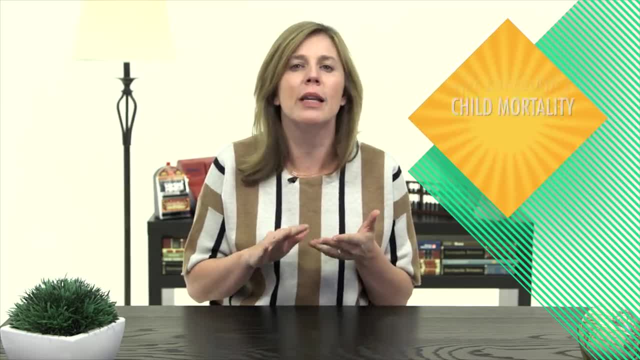 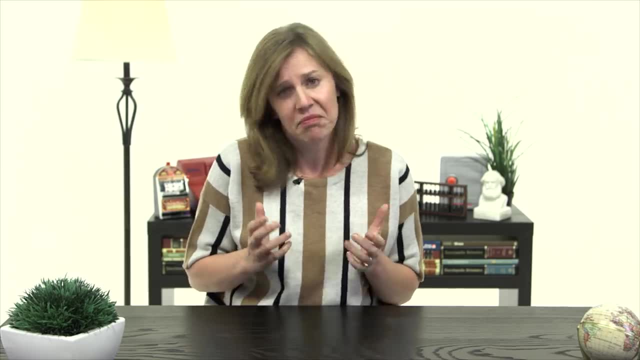 and throughout the ages. Using measurements like life expectancy, child mortality and income per capita, we can show the majority of humans that ever lived had terrible lives, Statistically speaking. It wasn't until the Industrial Revolution that people saw a significant and sustained 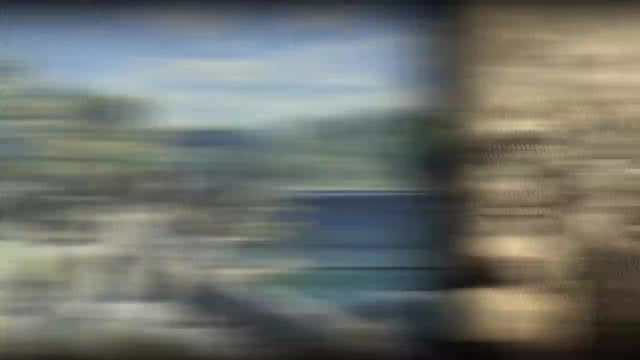 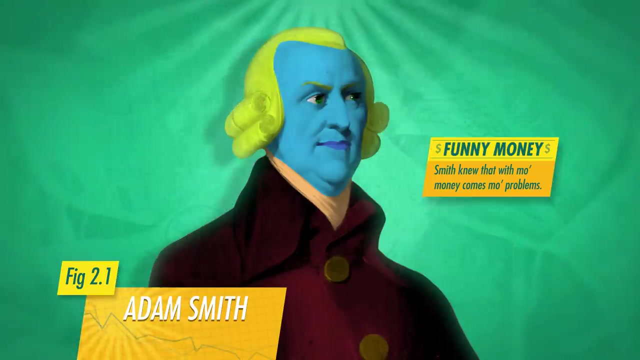 increase in their standard of living. Populations skyrocketed, but so did life expectancy and food supplies and hospitals and eventually toilets and refrigerators. It was in the beginning of the Industrial Revolution that Adam Smith, the first modern economist, wrote his book, An Inquiry into the Nature and Climate of the World. It was 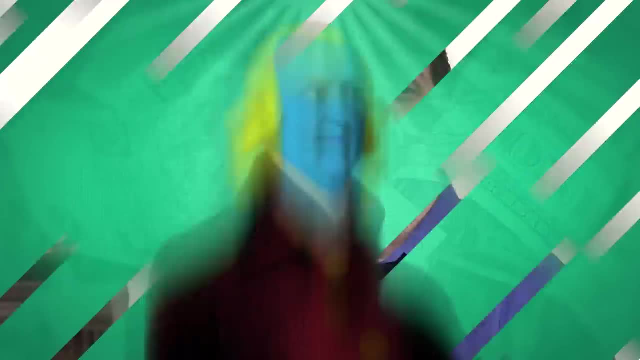 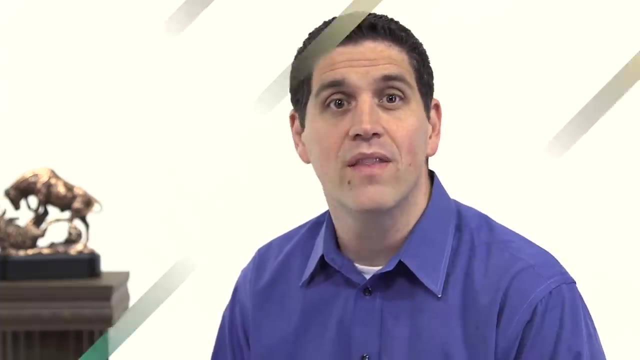 about the causes of the wealth of nations, or antikuntunkun. He wasn't great at naming books, but he was really good at explaining the source of prosperity. Smith concluded that it was specialization, what he called the division of labor, that made countries. 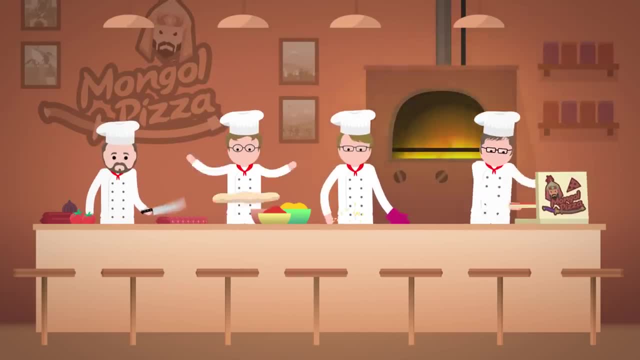 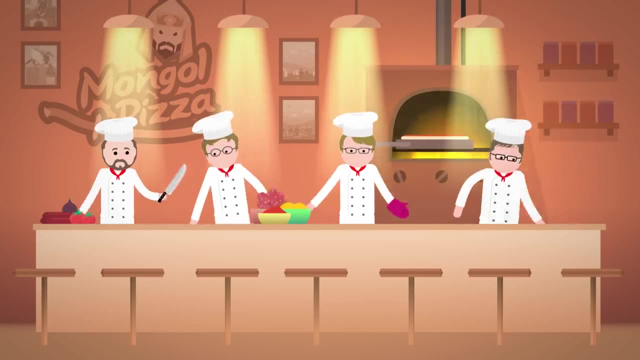 wealthy. Let's go to the Thought Bubble. When I think of specialization, I think of a pizza restaurant where different workers have specific tasks, like preparing the ingredients, making the pizza, putting it in the oven, taking it out and putting it in the box. This division of labor makes each worker more. 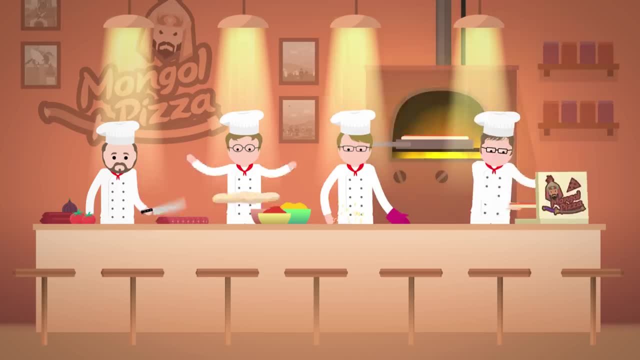 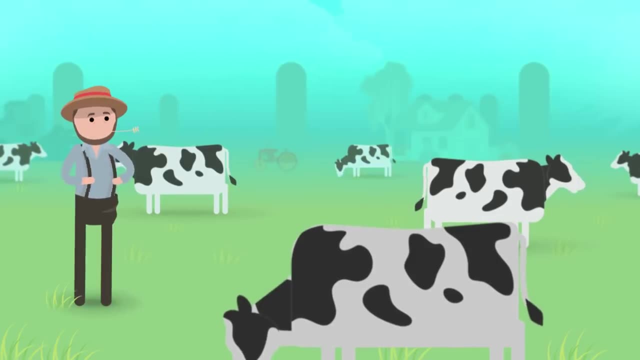 productive, since they can each focus on the thing they do best And they don't waste time switching between jobs. Specialization goes beyond the assembly line for pizza. To produce the cheese, there was a dairy farmer who specialized in raising cows. The oven was designed and manufactured. 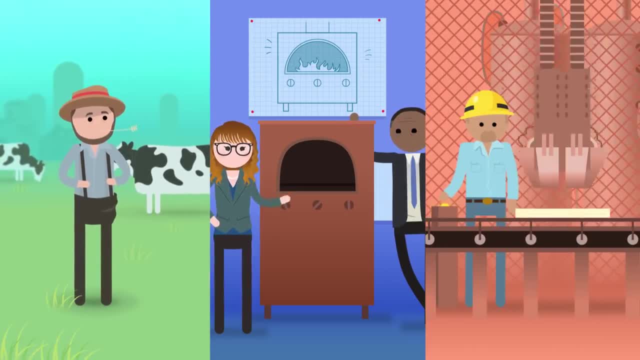 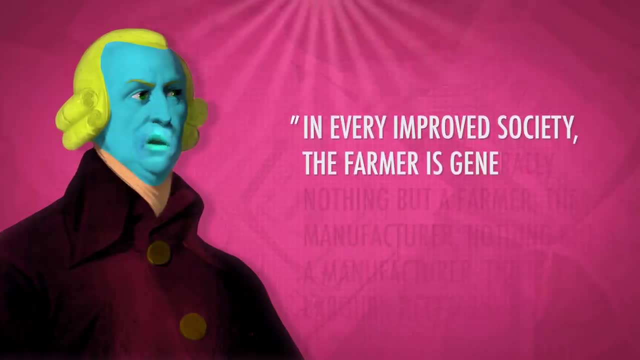 by people who specialize in engineering ovens. The friendly mustache guy in the pizza box. someone had to stamp him on there. I love that guy. Adam Smith observed: in every improved society the farmer is generally nothing but a farmer, The manufacturer nothing but a manufacturer. The labor necessary to produce any one complete. 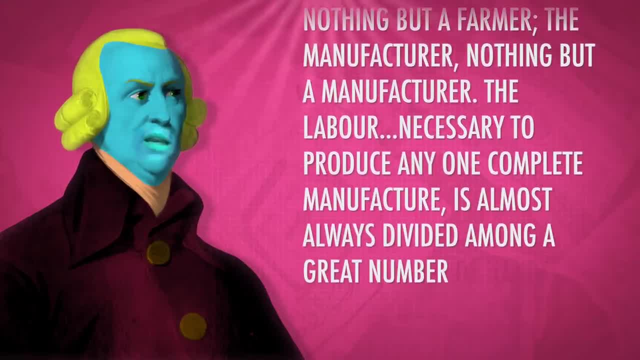 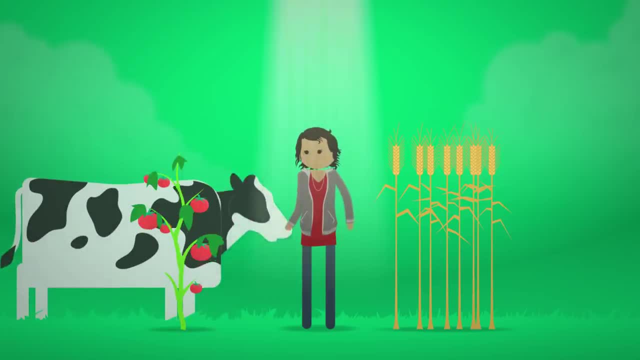 manufacturer is almost always divided among a great number of hands. Imagine what it would be like to make a pizza completely on your own, from scratch. You would have to grow the wheat and tomatoes and raise the cow. You would make the flour, the cheese, the oven, the pan and then draw the mustache guy on the box. Without specialization, 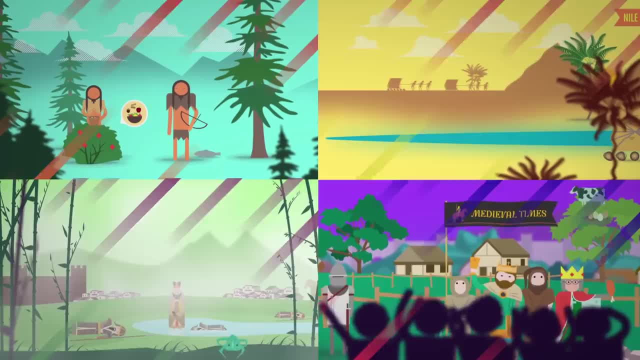 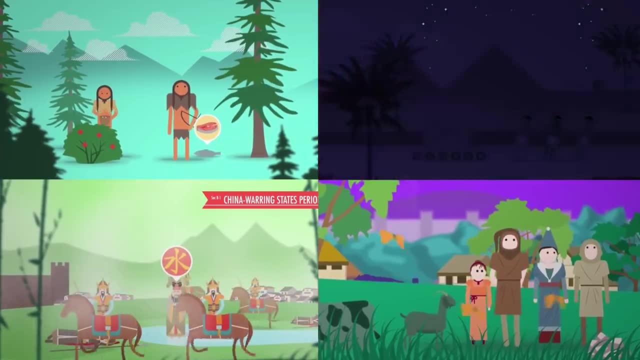 if you want something, you have to make it yourself, And for thousands of years of human history, specialization was well pretty minimal. Of course, humans specialized prior to the Industrial Revolution. It's one of the marks of civilization that we mentioned in our world history series. But the modern era has taken. 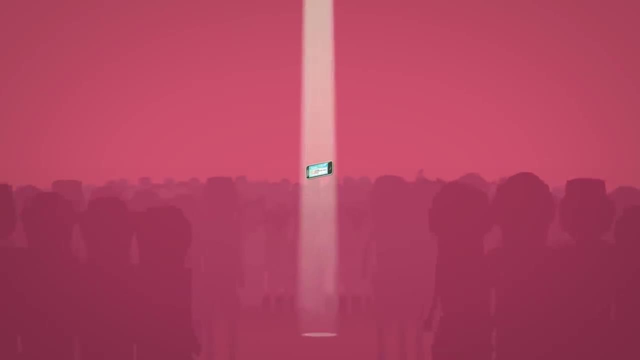 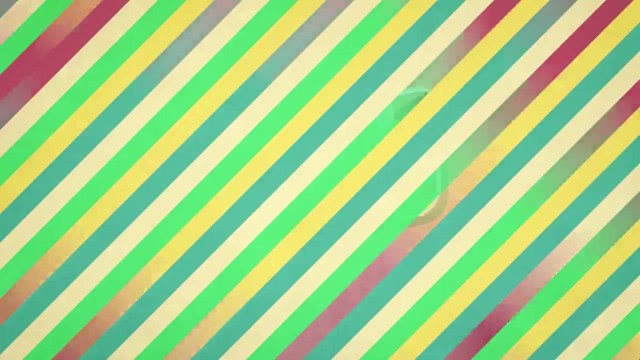 this to the extreme. Think of how many people, from how many different specialized fields, it takes to make a smartphone, all of them working in harmony. so I can tweet my super profound thoughts. Thanks, Thought Bubble. So specialization makes people more productive, But Adam Smith said that it's trade. that 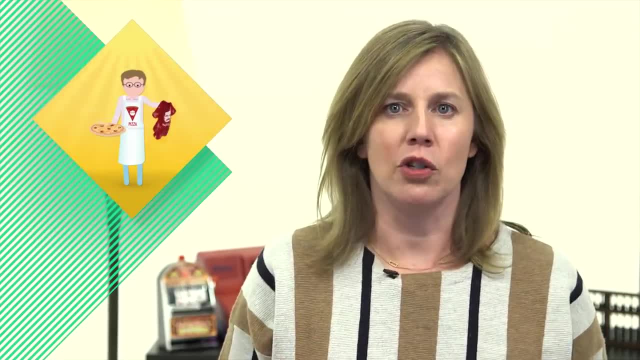 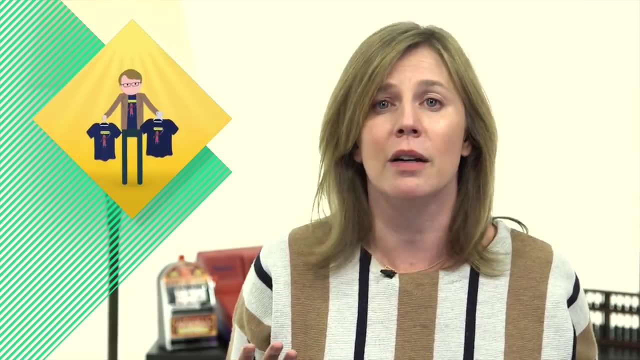 makes them better off. Assume that John can produce either pizza or t-shirts. If he's way better at producing pizza, then he should specialize in making pizza and then trade with someone else like Hank, who's way better at making t-shirts. Everyone knows Hank's. 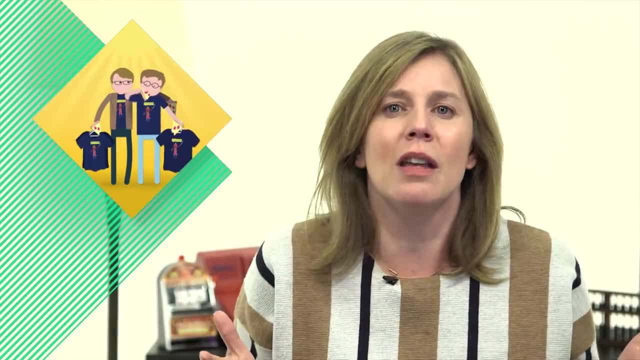 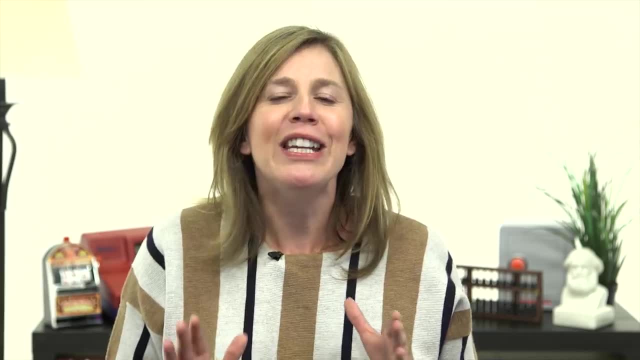 better at making t-shirts right With trade. each of them can end up with more pizza and shirts than if they tried to make them on their own. To fully explain this idea of the benefits of trade, we need to show you an economic 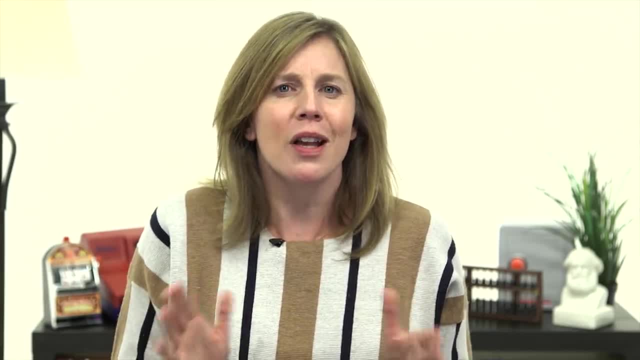 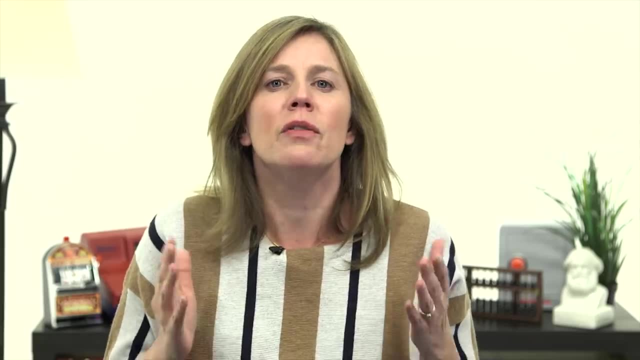 model. But before we go any further, know that economists geek out over models and graphs. Don't get all worked up about the numbers. They're not that complicated. Models are just visuals to help us simplify and explain concepts. It's time for the model, so let's. 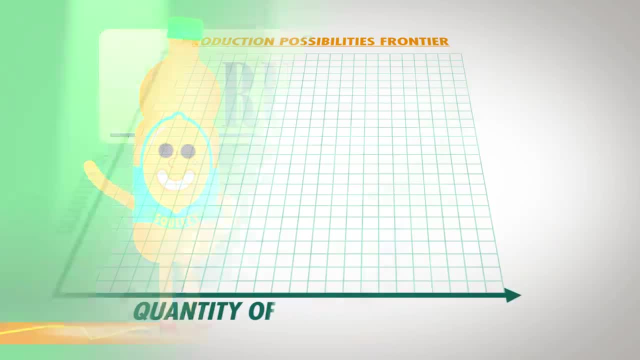 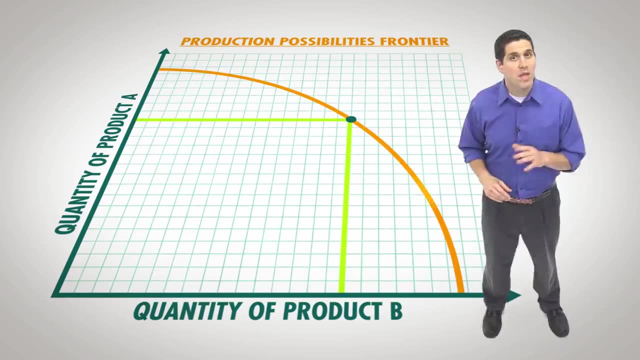 go to the runway Now. this is the first graph you'll see in an economics textbook. It's called the Production Possibilities Frontier, or PPF. The PPF shows the different combinations of two goods being produced using all resources efficiently. Now here's a made-up example. 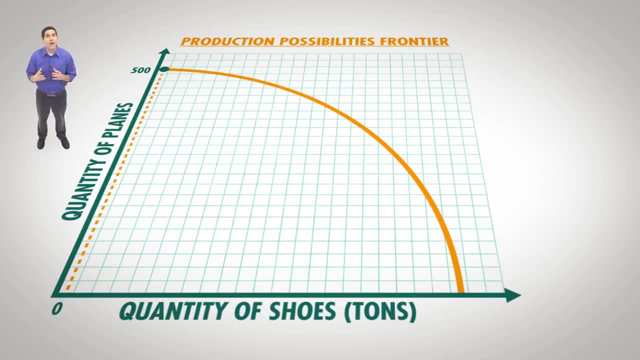 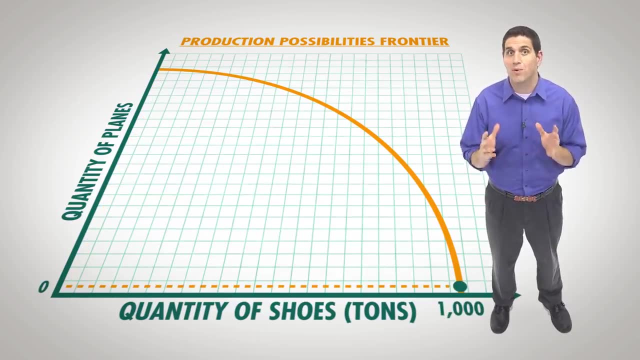 If the United States uses all of its workers and factories to produce airplanes, it can produce 500 per day, but it can't produce any shoes. Now, if they use all their resources to produce shoes, they can produce 1,000 tons per day, but they can't produce any planes. 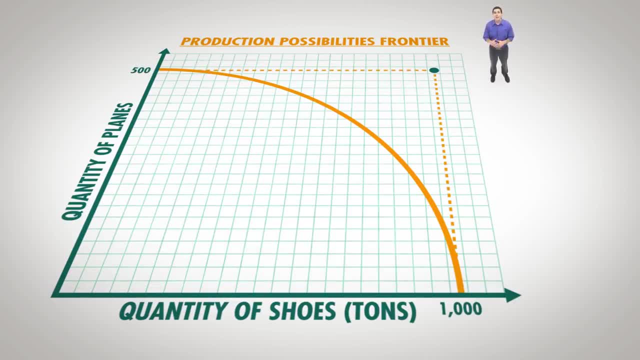 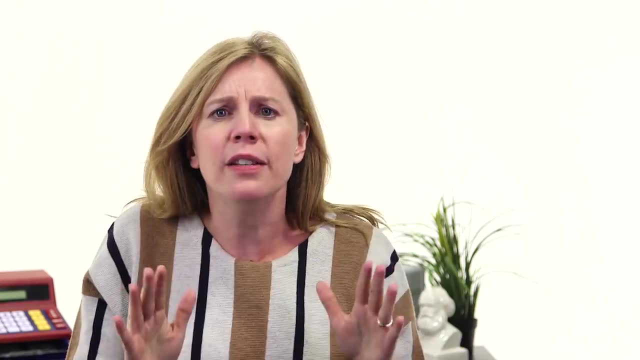 Now, because the United States has limited resources, they can't produce any combination beyond the Production Possibilities Frontier. So it's impossible to produce 500 planes and 1,000 tons of shoes. Wait, wait, wait. Mr Clifford, I want to stop you here for a second. We don't live. 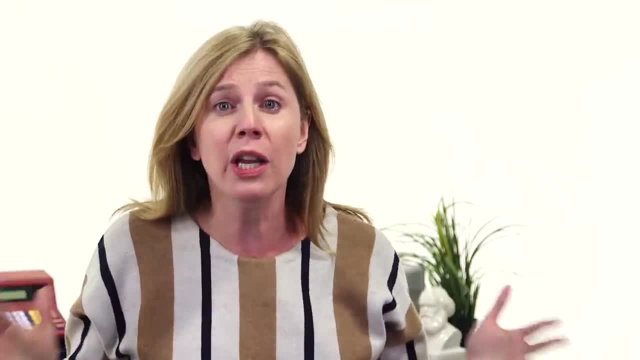 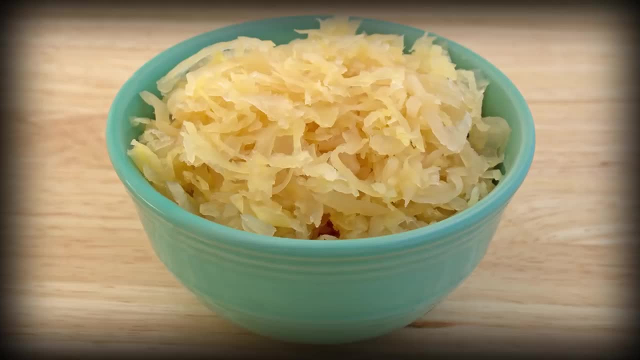 in a world where there are only two things that a country can produce. There are like a million things that US workers can choose to make: Toilet paper, zippers, adorable stuff, kitty cats holding heart, artisanal sauerkraut. We don't live in a world of just shoes and 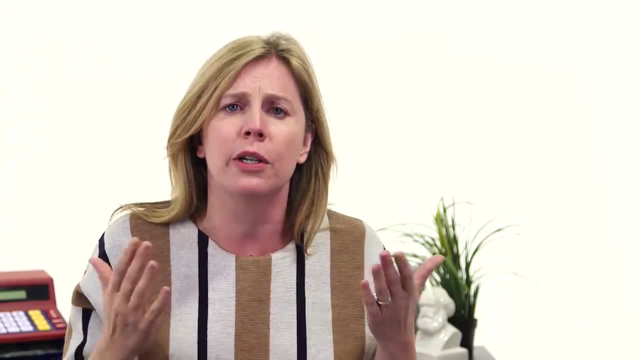 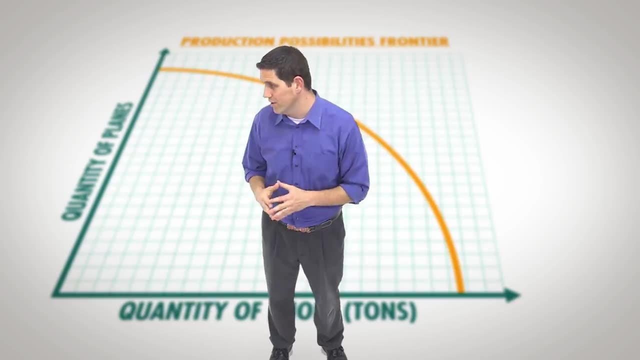 airplanes. So what's the real-world value of the Production Possibilities Frontier? The idea is, once you really understand that there's trade-offs between producing two goods, that same logic applies to any number of goods, And adding additional goods makes it more complex but doesn't really add any more insights. 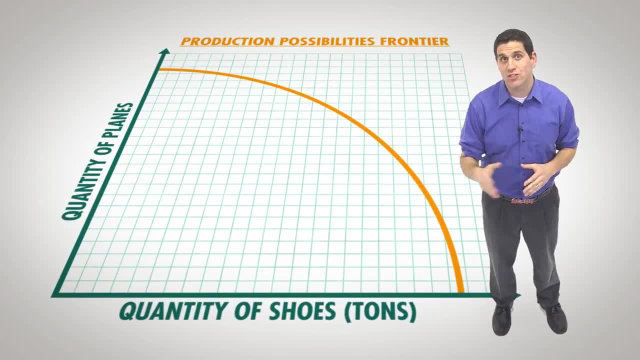 So economists usually stick with just two goods. Now, what if American companies mismanaged their resources and tried to produce planes and shoe factories, and shoes and plane factories? Well, they'd be at a point inside the Production Possibilities Frontier, showing an inefficient use of resources. 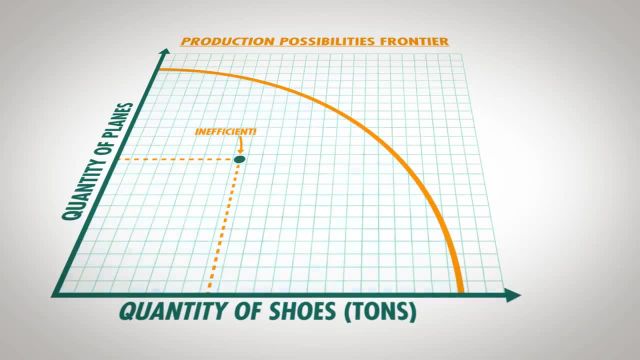 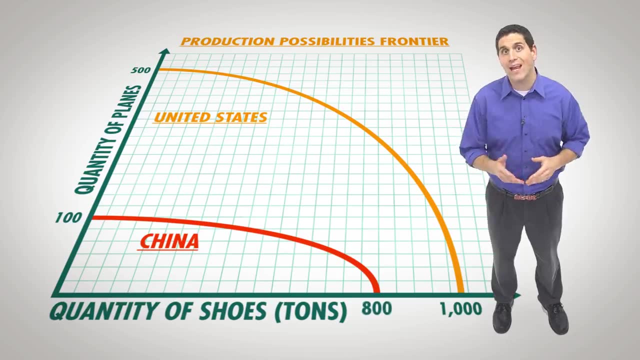 So every possible combination inside the curve is inefficient and on the curve is efficient and outside the curve is impossible. Now let's compare this PPF to China's. China can produce 100 planes per day or 800 tons of shoes. 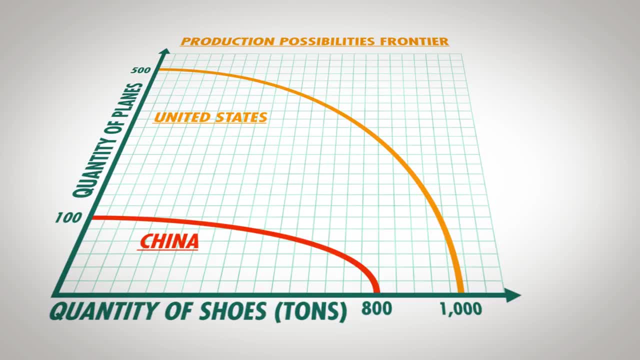 Now, if the United States can produce more planes than China, they have an absolute advantage in the production of planes. The US also has an absolute advantage in the production of shoes. Since the US can produce more of both goods, you might think there's no reason to trade. 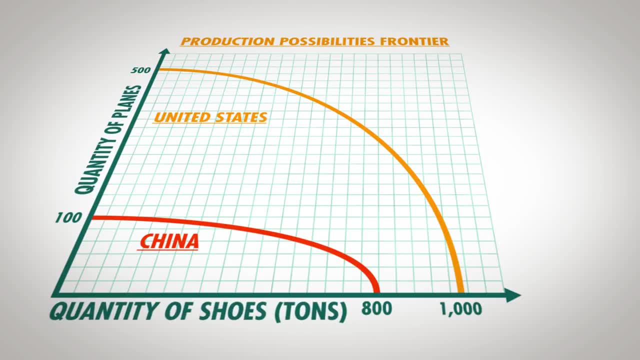 but they should just produce both on their own. Well, no, Remember, specialization in trade makes people, and in this case countries, better off. Now stick with me. Let's calculate the opportunity cost for the United States to produce one plane. Every single time they produce an additional plane, it costs them two tons of shoes. 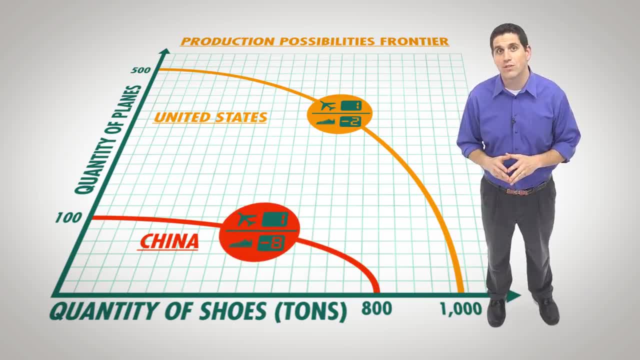 China, on the other hand, gives up eight tons of shoes for each plane they produce, And since the US has a lower opportunity cost, they can produce more. And since the US has a lower opportunity cost, they have what's called a comparative. 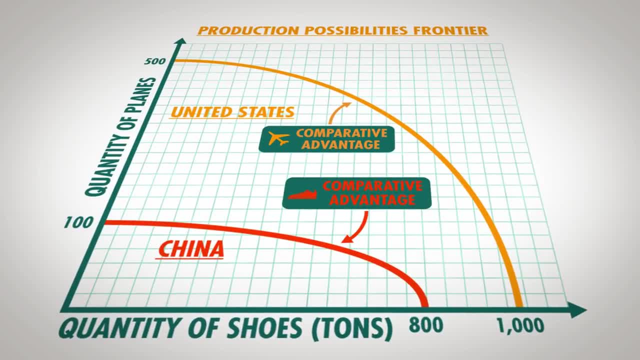 advantage. China has a comparative advantage in the production of shoes. But here's the best part: If the US specializes in planes, they can import shoes from China at a lower opportunity cost than if they produce shoes themselves. For example, if these two countries make a deal to trade one plane for four tons of shoes. 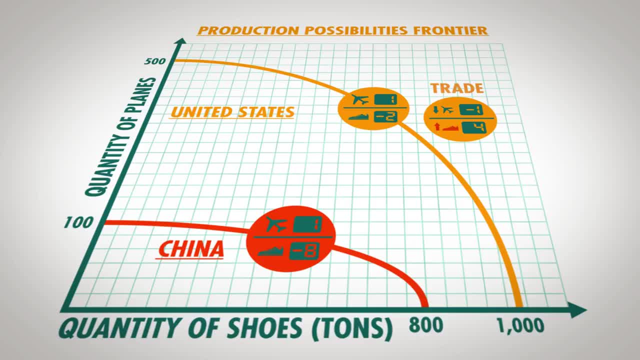 the US would be better off. They would rather get four tons of shoes per plane from China than only get two tons of shoes per plane by making shoes on their own. Now, China is also better off. They would rather trade four tons of shoes for a plane. 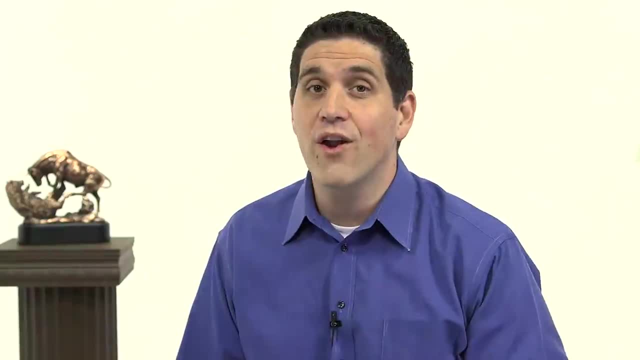 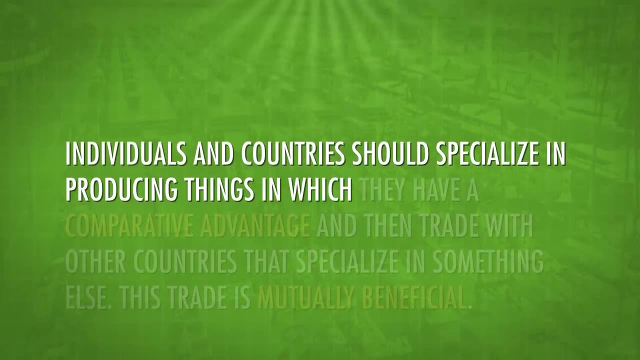 than give up eight tons of shoes for producing a plane on their own. Now, hopefully, your head isn't spinning. Being able to do these calculations is good, but it's more important to understand the main idea. Individuals and countries should specialize in producing things in which they have a comparative. 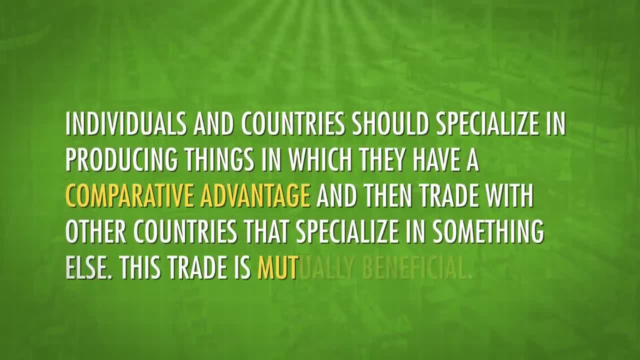 advantage, and then trade with other countries that specialize in something else. This trade is mutually beneficial. Now that's the production possibilities frontier In the real world. it's way more complicated than the simplified model, and we're only in the beginning. 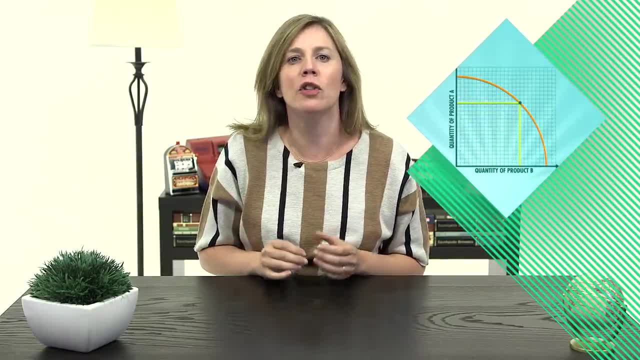 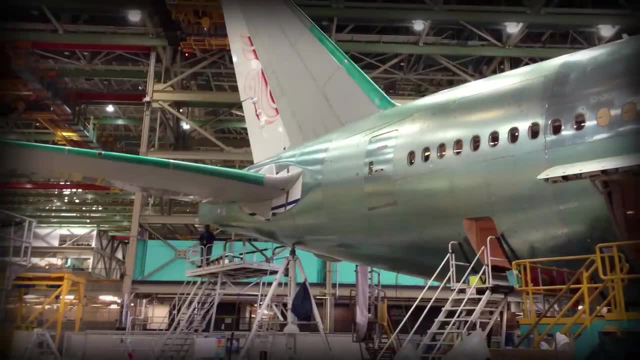 So this graph is super simplified, but the idea that countries should focus on producing the products for which they are better suited is huge, Way huge. In reality, the US is the world's leading producer of shoes. The US is the world's leading manufacturer and exporter of airplanes. 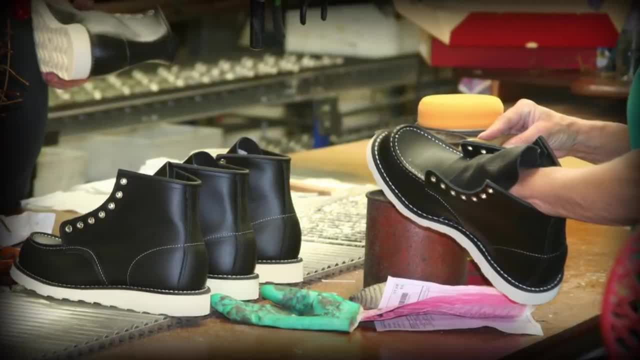 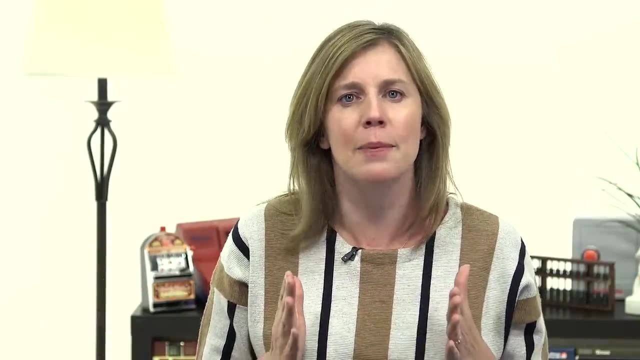 It produces more than 40% of all planes. At the same time, the US produces less than 2% of the world's shoes, electing instead to import them from countries in Asia. The graphs aren't real, but the concepts are. 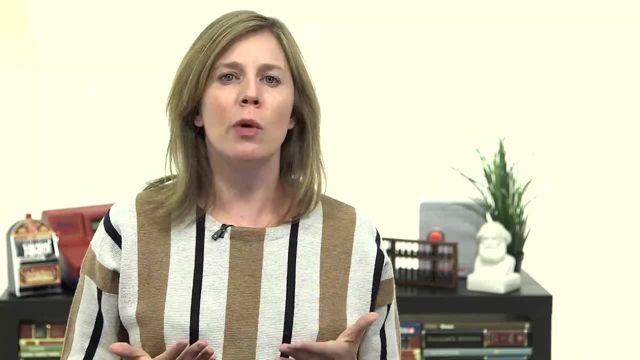 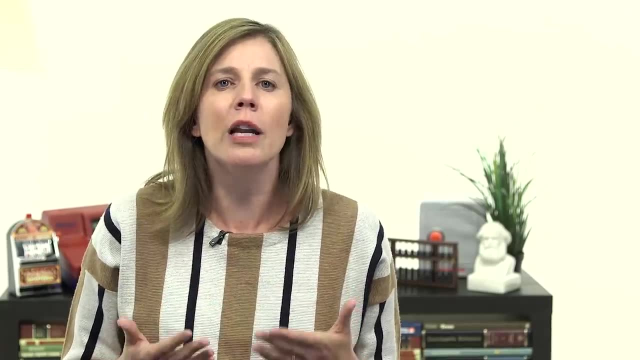 Another reason you should learn this is because you might hear a politician or someone on the news argue that international trade destroys domestic jobs And, even though it may seem counterintuitive, economists for centuries have argued that trade is mutually beneficial to whoever's trading. 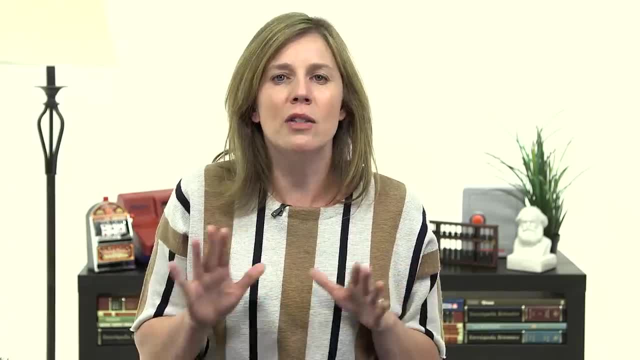 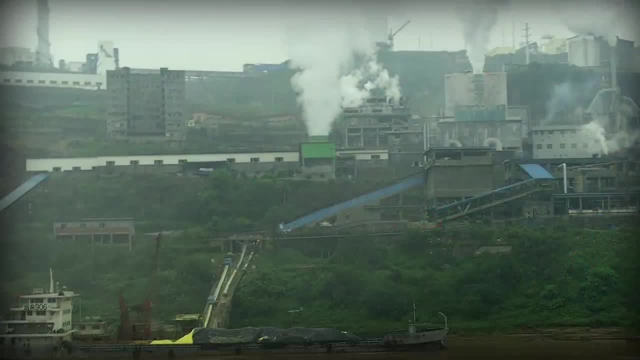 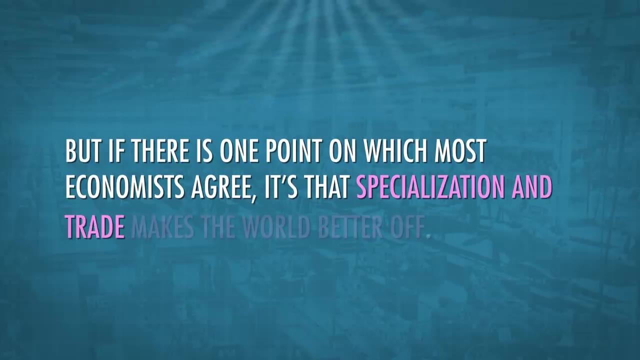 Now you know why. Now, to be fair, there are all sorts of other intolerable issues associated with international trade, like child labor, dangerous working conditions and pollution, And we promise to address these in a future video. But if there's one point on which most economists agree, it's that specialization in trade. 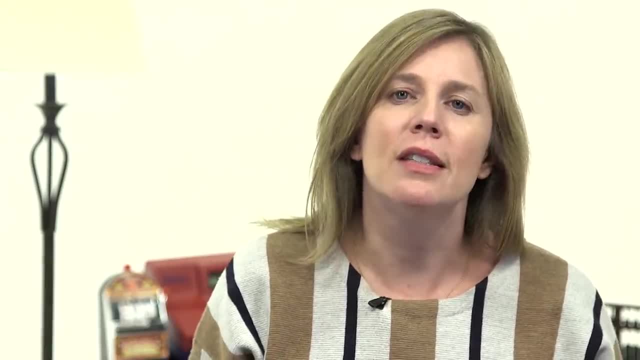 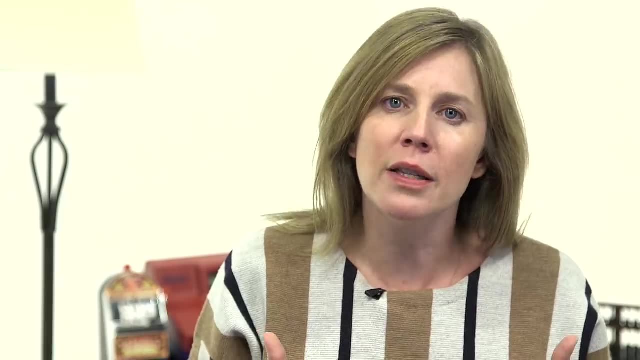 makes the world better off. No country in recent decades has achieved sustained improvements in living standards without open trade with the rest of the world. Countries like Cuba, Venezuela, Zimbabwe and Iran that are voluntarily or involuntarily cut off from the world. remain less economically developed than they could be. On the other hand, countries that have opened their doors to trade, like Japan and Taiwan, or, more recently, China and India, have seen massive improvements in their standards of living. Adam Smith was on to something.